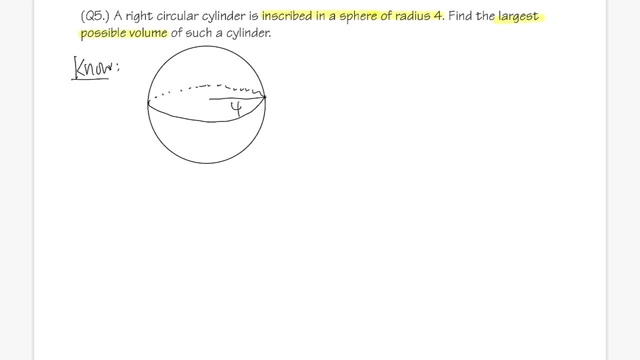 of four. So this right here is four. Now we want to just kind of construct a cylinder inside So you can put a cylinder like this, Just make a horizontal cut and then like a vertical cut And then somehow you make a cylinder like this And you can imagine, if you make the cylinder like this they will have different volumes. So let's just take a look at the blue one and 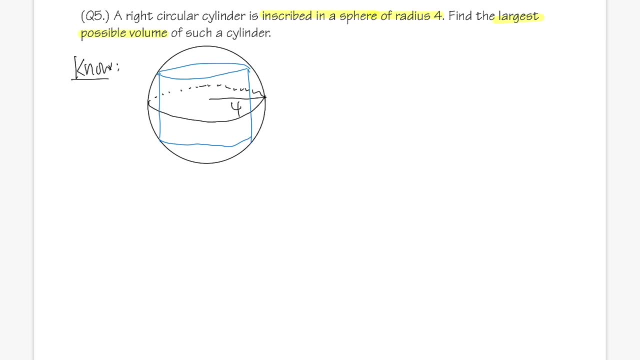 try to see what we can possibly do with this. All right, I will have to remind you guys that. So let me just remind you. note, when we have a volume of a cylinder, when it's a circular cylinder, this right here is pi r square h right And the cylinder is the circular cylinder, like that. 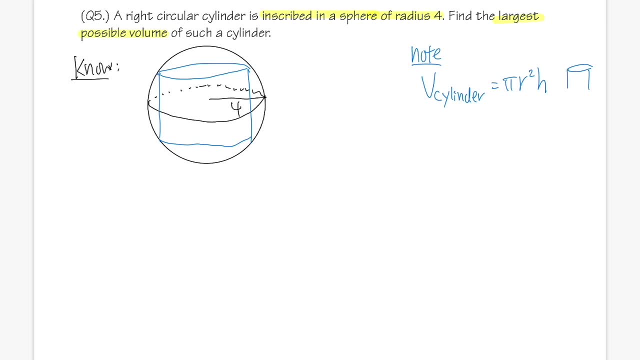 So one of the formulas that you should definitely remember for optimization, also related rates. Let me just write this. Okay. so, based on this, what do we know, though? That's it, huh, And what do we want to know? Well, we do want to know the volume of the cylinder, and we want it to be the smallest. we want to be the biggest possible cylinder. 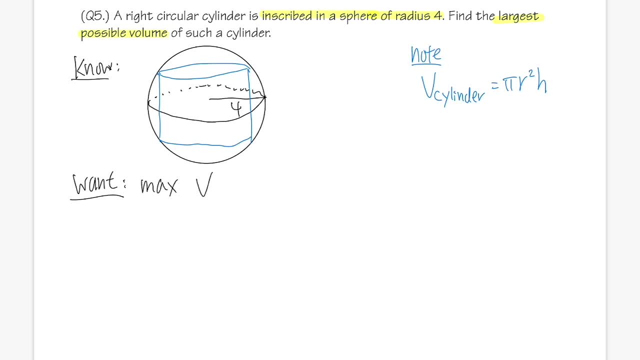 So we want the maximum of the volume of the blue cylinder. So how can we do it? Well, it looks like we need to have the r. we don't have the r yet and we don't have the h yet, But don't worry, this is how we do the math Here. let's take a look at the sphere. If you just look at it from one side, then that's called the cross section, which is just going to be a circle, And then 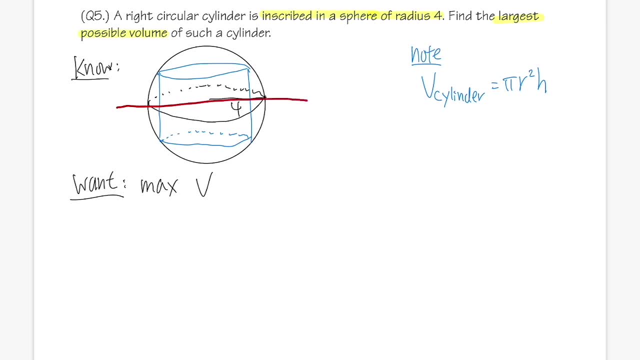 if you put the x and y axis, like we usually do when we do calculus and even physics, we will put a x, one axis. So let's say, this is the x axis and this is the y axis. All right, Now what does this do? In fact, this right here will turn the question, like what we did earlier. Yeah, do you see it? this picture? and 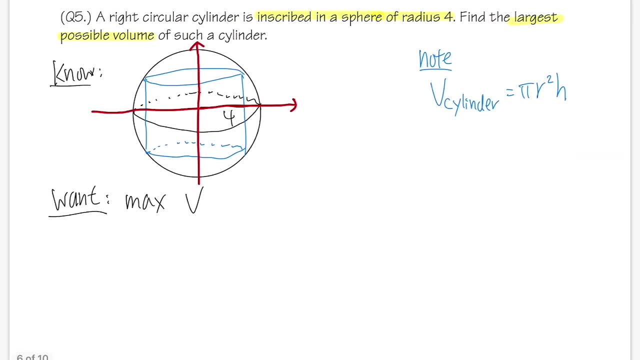 this picture. Here we also need to know the equation of the circle, And the equation of the circle is: x minus h, squared, plus y minus k squared, equals r squared. Our center is at 00.. So we just have x squared plus y squared, equals r, which is four, and we square that. So that's the equation of the circle. Now we want the radius that we're talking about. 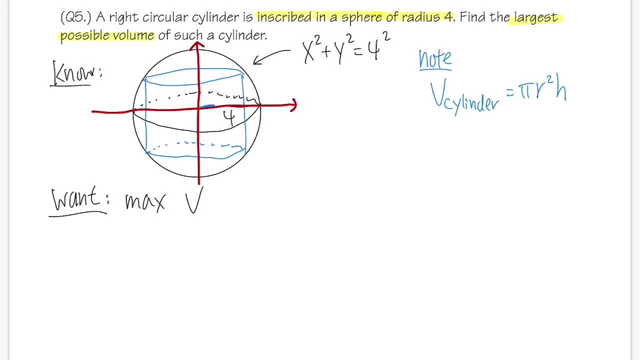 earlier. From here to here it's the radius of the cylinder. I don't know what that is. I'll call that x, And from here to here it will be the height of the cylinder, but not really technically the y, because I'm putting down the x- y plane like that right. So here's the deal Based on our labeling. 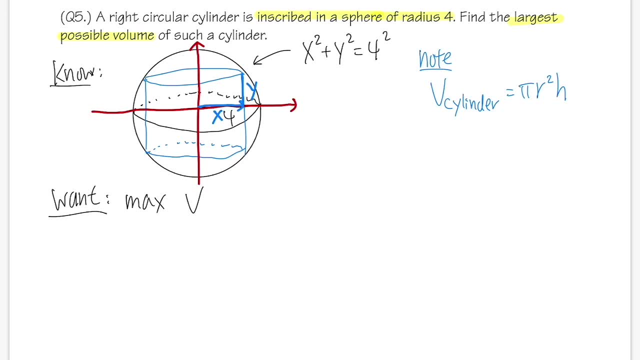 our volume of the blue cylinder is pi And then the radius is x. So we'll just multiply by x And we square that, because that's the radius squared And we want the whole height right? remember the height it's from here to here. it's two y by symmetry: On the top is y, the bottom will also be y, So the whole thing is two y. So multiply by two y. 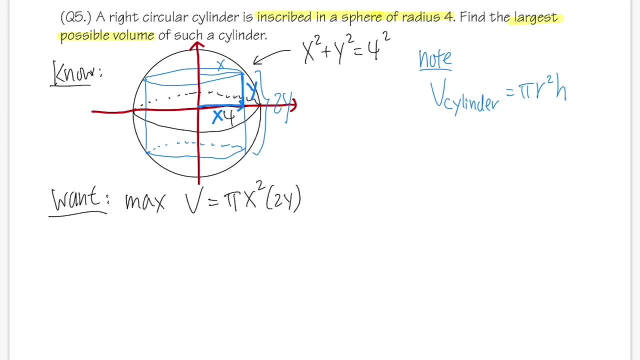 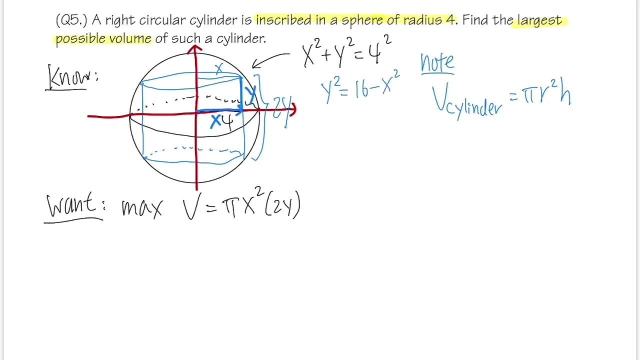 All right, so that's that. The trick is, you will have to look at this as a cross section and also recall the equation of a circle. Now, same thing. Here we have the y- So perhaps let's go here- and minus x squared on both sides, So we get: y squared is equal to four squared, which is 16, and then minus x squared, And then just take the positive square root, So y is equal to the square root of 16.. 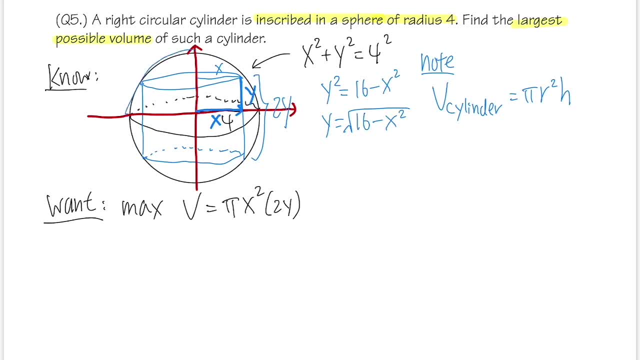 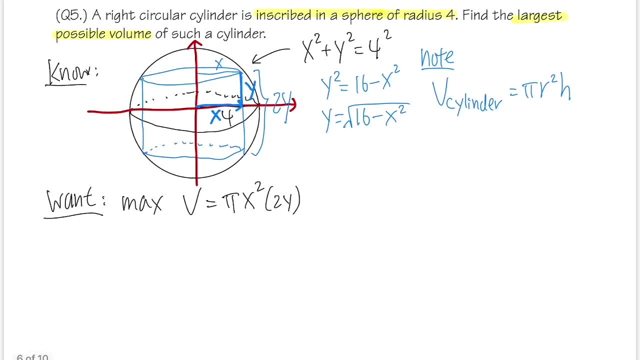 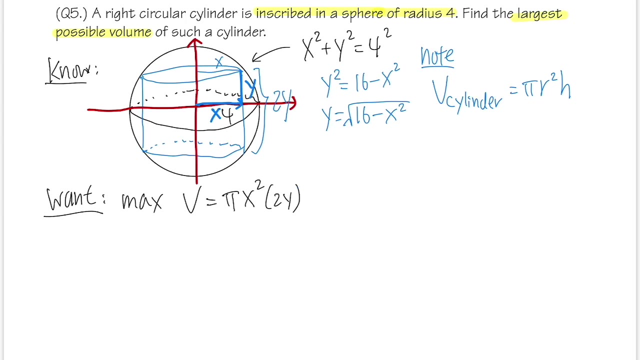 Minus x squared, because, based on our picture, we just want the y to be on the top right here And if you have a negative you end up with a negative volume. So just positive square root is okay, And then we'll put this right here. That will give us the volume in terms of just x. And let me write down the two first. So we will have two pi and then x squared, and then for the y, which is that square root. 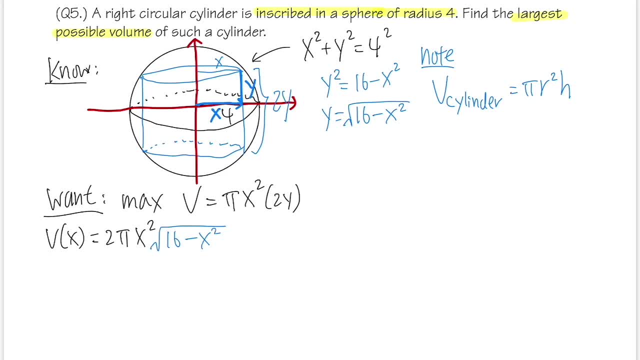 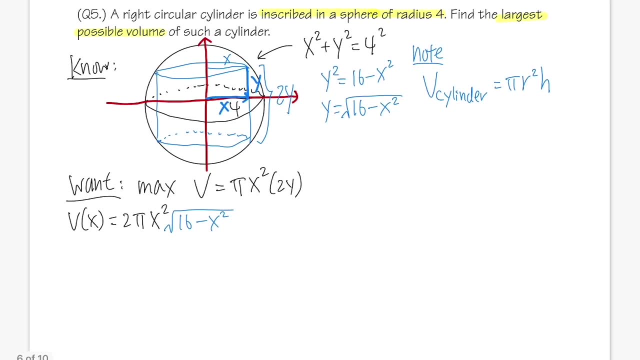 A square root of 16 minus x squared, And unfortunately we cannot really do any algebra to simplify this expression, So we'll just have to do calculus now And we will have to use the product rule. So go ahead. I will look at this as the first function. So we will have two pi x squared times. the derivative of the second. The derivative of the second is the square root is. we will have the 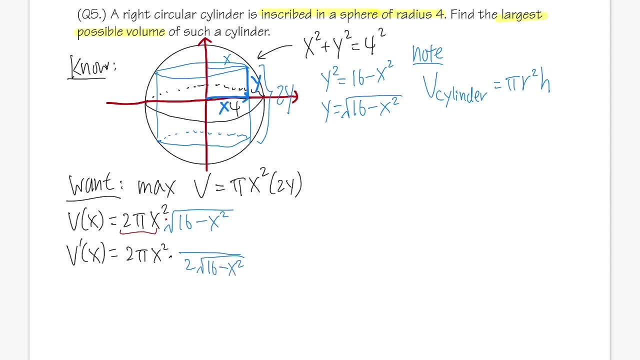 over two square root of 16 minus x squared. And don't forget the chain rule. So multiply by negative two x, And then we are going to add the second function, which is the square root 16 minus x squared, and then multiply by the derivative first. For that we just have to do the power rule. for this, Bring the two to the front. we give four pi and then x to the first power. That's that, And then perhaps we can clean things up. 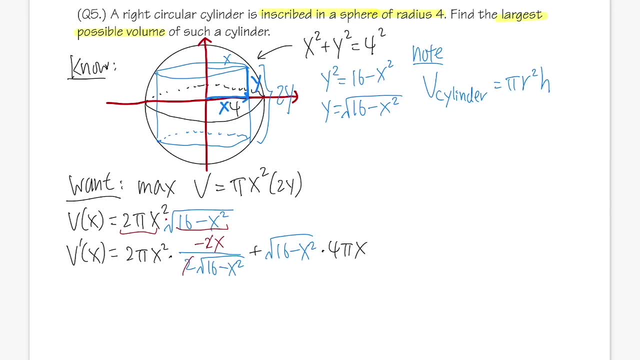 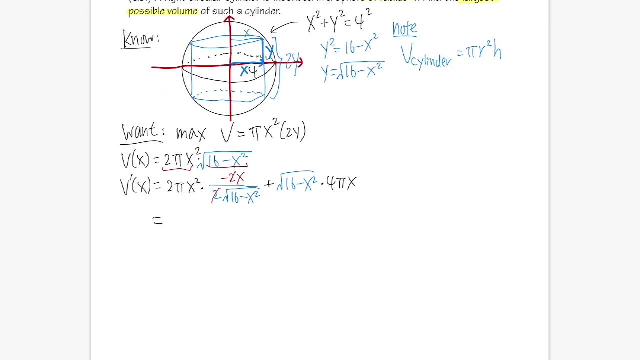 A little bit. Two and two- cancel. That's about all. And then I'm just going to rewrite this. This is again our first derivative. So x squared times x, we have x to the third power And that's a negative here. So we have negative two pi x to the third power over square root of 16 minus x squared. And then for the other part, let's write it as plus. 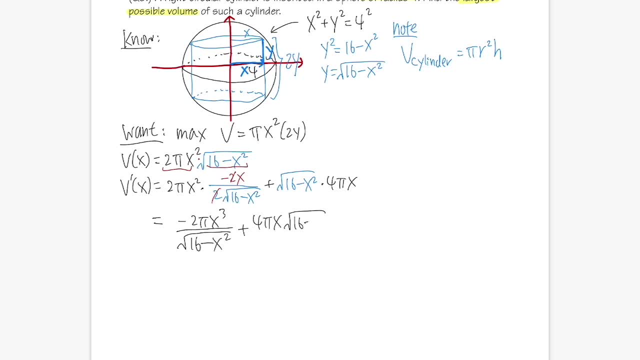 Plus four pi x times the square root of 16 minus x squared. Let's get the common denominator: Multiply the top and bottom by square root of 16 minus x squared. So that means we get both of them being dividing square root of 16 minus x squared, And for the first part we have negative two pi x to the third power. 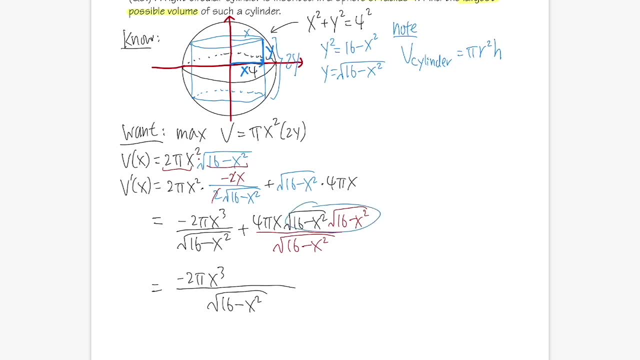 And then we see that this and that, multiplying, we will just get 16 minus x squared. And then take this, distribute it, So four times 16, we get plus 64, and then the pi x, and then four pi x times that is minus four pi x to the third power. 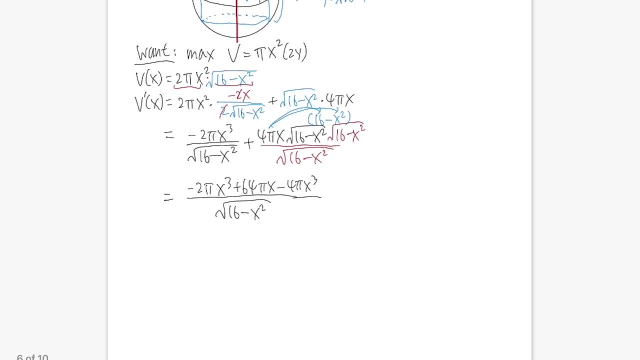 And we have two more things that we can do. right, Combine this and that to these two things, So we get negative six pi x to the third power, plus 64 pi x over square root of 16 minus x. squared A lot, huh. And now go ahead and set this to be zero And in fact you don't need to worry about the critical number when the derivative is not. 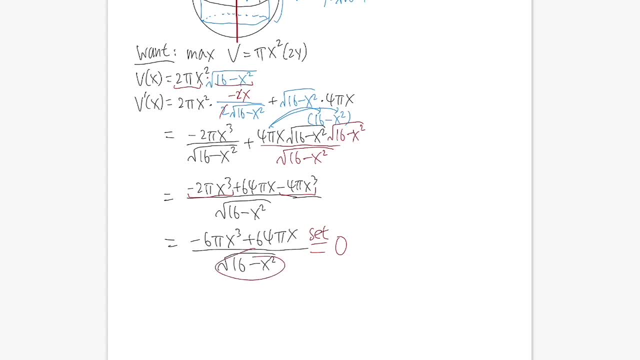 defined, because that's the case when x is equal to four, because when you plug in four into the following equation you get zero for the volume. So you don't really have to worry about that. That being said, just worry about where the derivative is equal to zero, which is just the top being equal to zero. So we look at negative six pi x to the third power, plus 64 pi x being equal to zero. 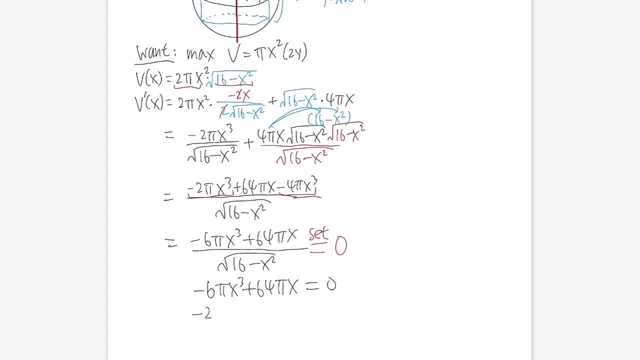 To solve this equation, let's go ahead and factor out negative 2 pi x, so we will get 3 x squared minus 64, divided by 2 is 32 and the pi x are out already and we have critical numbers. when this is equal to zero, that means x is equal to zero. 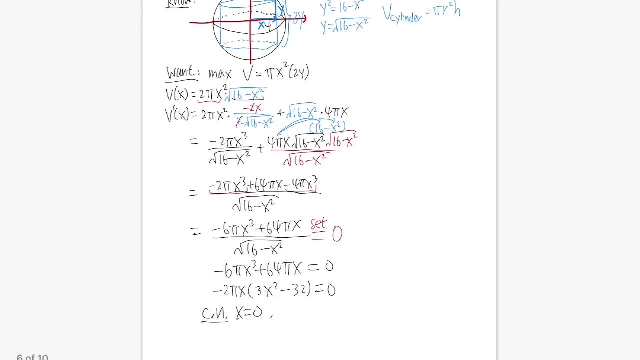 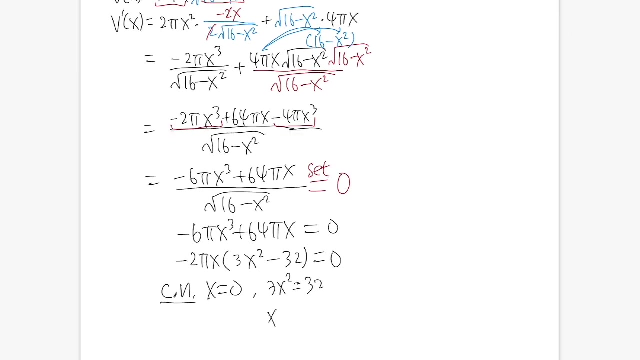 but we don't care about this seriously because that will give us zero for the volume. and we care about 3 x minus 32 is equal to zero, which is 3 x squared equals 32, and then we can divide both sides by 3. take the square root so we get: x is equal to. 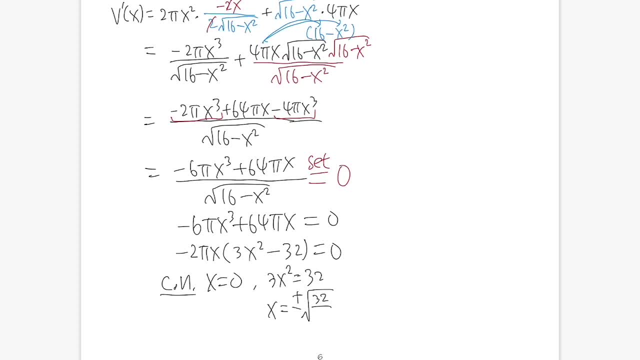 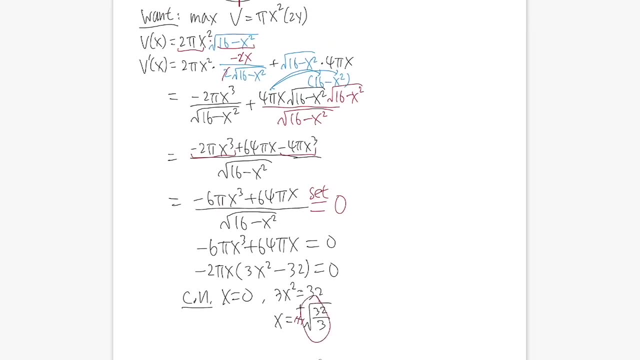 plus or minus square root of 32 over 3, and of course, we are just going to get rid of the negative. and now, of course, you know this is going to give us the answer, but i will still provide a quick example of how to do it. so let's go ahead and factor out negative 2 pi x squared minus 32. 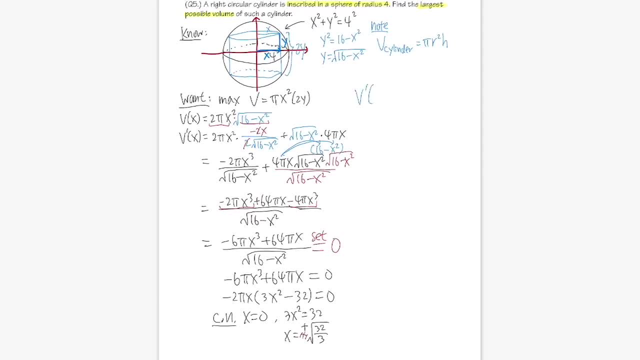 the derivative at square root of 32 over 3. and notice, i didn't simplify this because you guys will see why the derivative is zero and i will just do the first derivative test because i don't want to take the derivative. that again. all right, i will just show you like this: 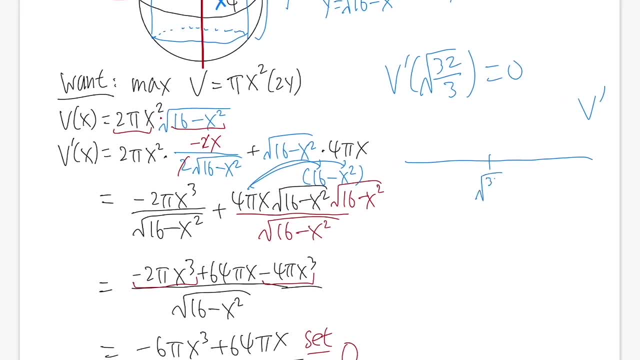 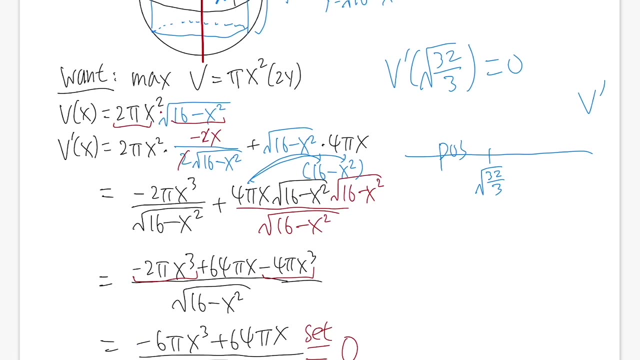 the derivative at here is zero. and if you put the derivative at here, when you put the number less than this into the derivative, i will tell you you will get positive derivative right before it. and if you put a number slightly bigger than this into the derivative, you will get negative. 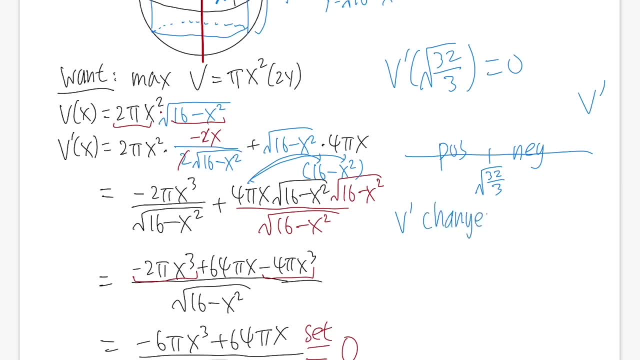 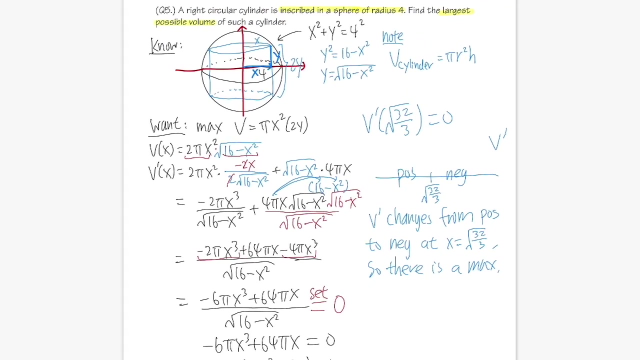 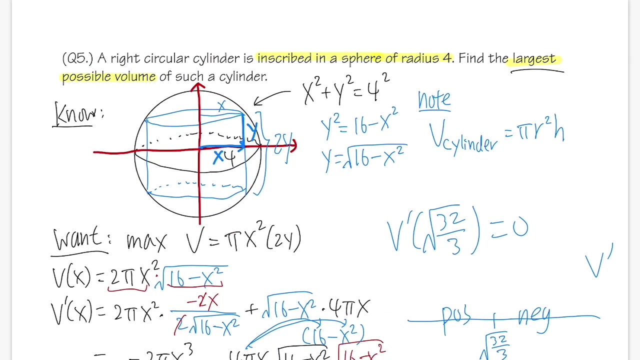 so, as we can see, phi prime changes from positive to negative. x equals square root of 32 over 3, so there is a maximum and this is called the first derivative test. and yeah, it shouldn't actually be okay. now we are going to answer the question and it's only asking us to get the largest possible volume. 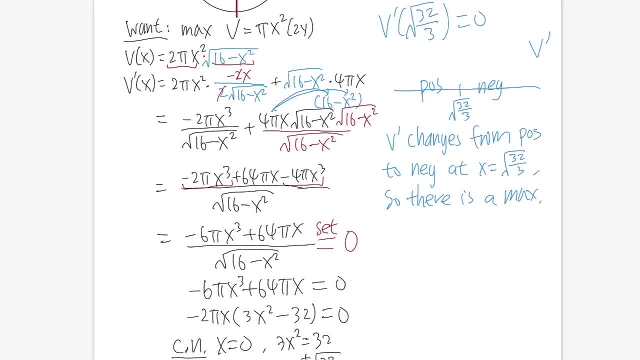 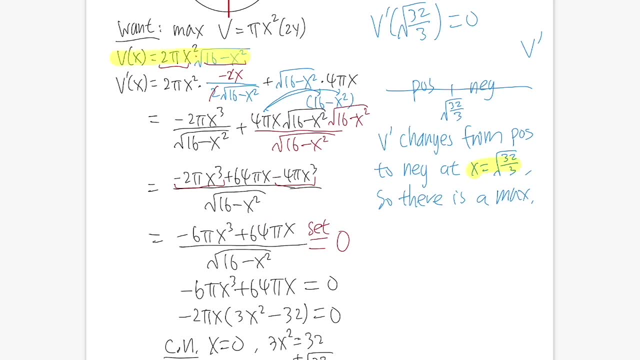 so i don't need to give the dimension, i will just plug in the critical number, which is this, right here into our volume equation. so, as we can see, we will get volume of square root of 32 over 3. that is just 2 pi times x squared, which is, you know, the square root and the square will. 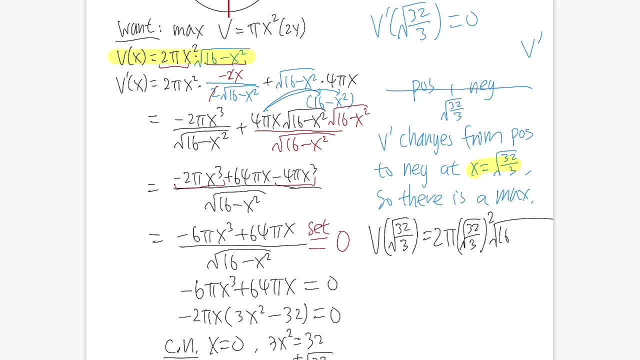 cancel each other very nicely. that's why i didn't simplify. but anyway, square root: 16 minus x right, which is 32 over 32 over 3 squared, and now let's just go ahead and do the work. so this right here is equal to 2 times pi. 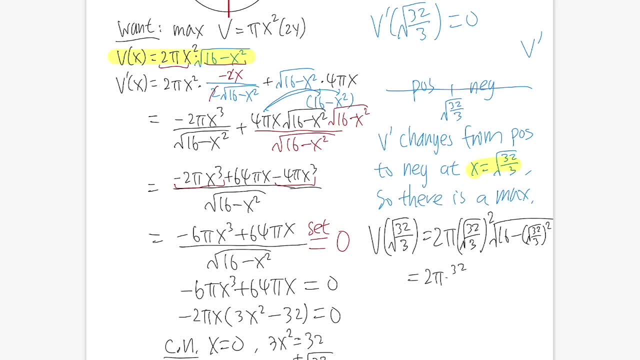 times square root and the square cancel, so 32 over 3 times. okay for the inside here, go ahead and just work it out on your own. it's just 16 minus 32 over 3, which is 48 over 3 minus 32 over 3, which we get 16 over 3, and 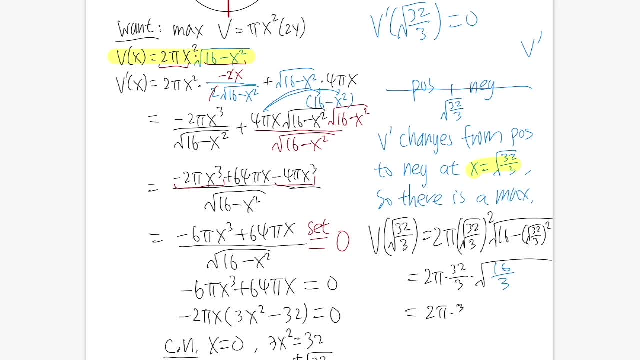 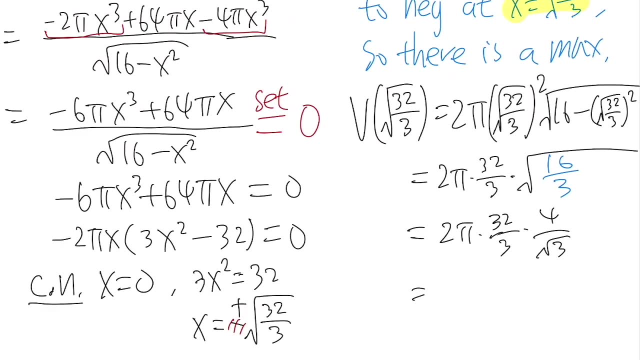 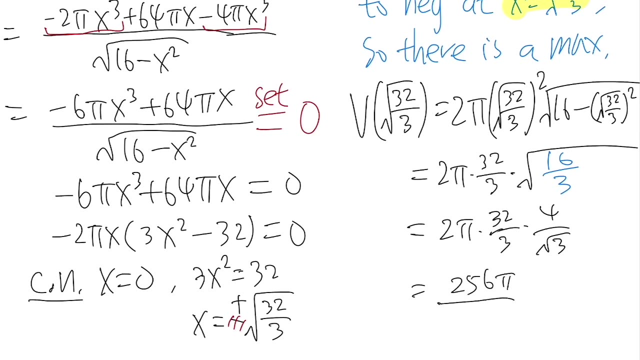 this right here will be 2 pi times 32 over 3 times 4 over square root of 3. so all in all, 4 times 2 is 8, 8 times that is 256 pi over 3 square root of 3, and this right here will be the answer.